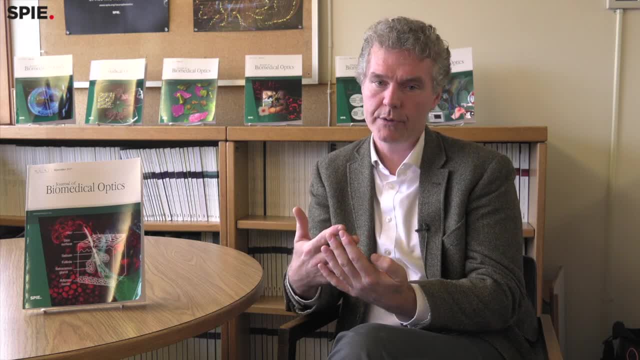 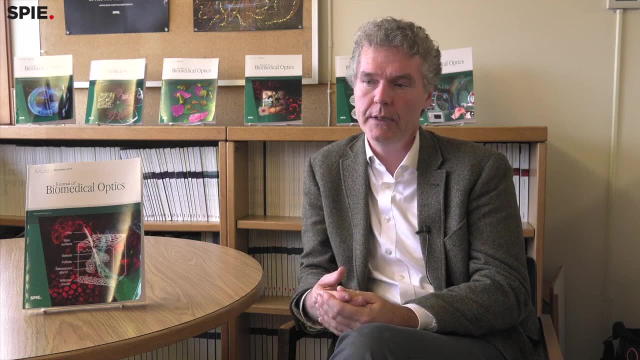 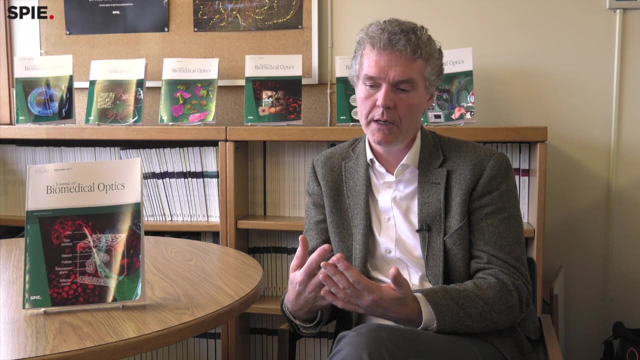 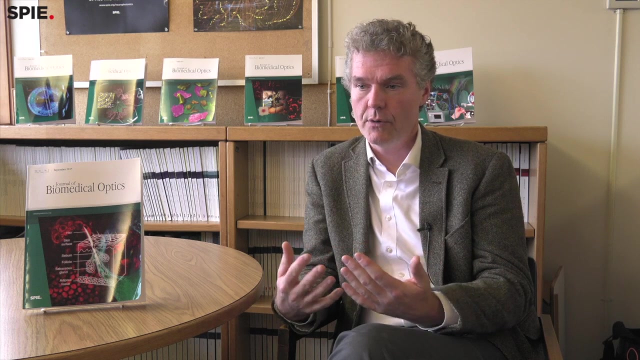 the needs in medicine and the technologies being produced by engineers and physical scientists. It's that intersection that is the journal, the scope of the journal, And so it's intentionally broad and intended to catch papers from both those sectors, and with the focus on translation, I think, more and more as the journal has grown and matured. 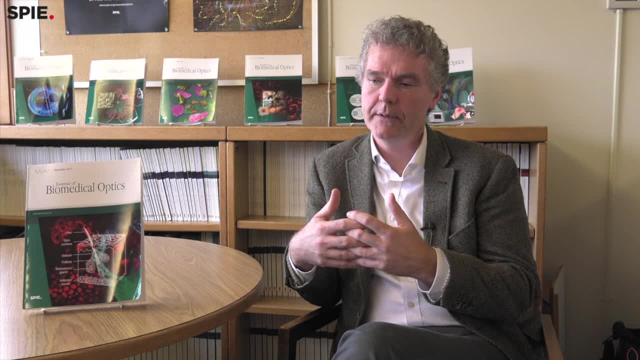 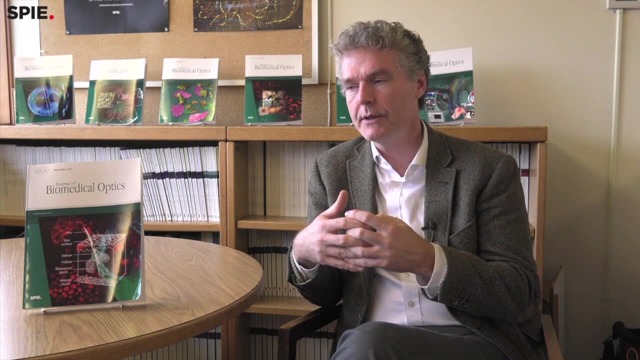 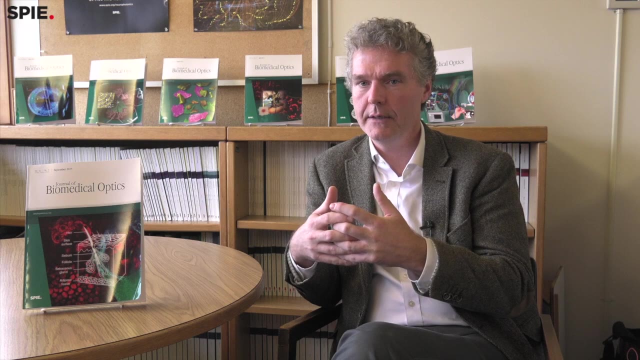 it's a little bit more of a cross-section of the journal, But making that connection is one of the things that I would like to do: Having industry a little bit more involved- as involved as they can be in publishing, And having academics be a little more responsive and connected to industry so that 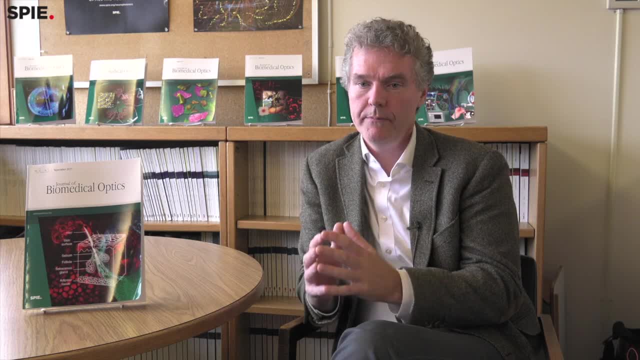 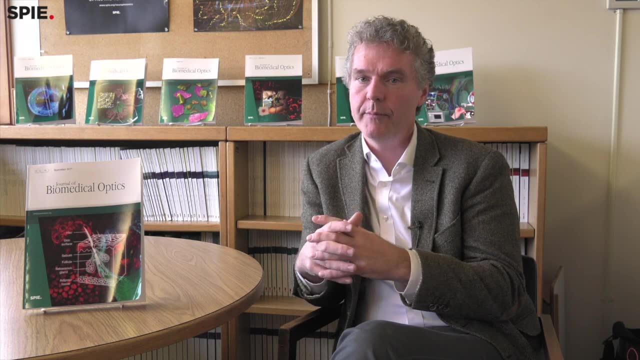 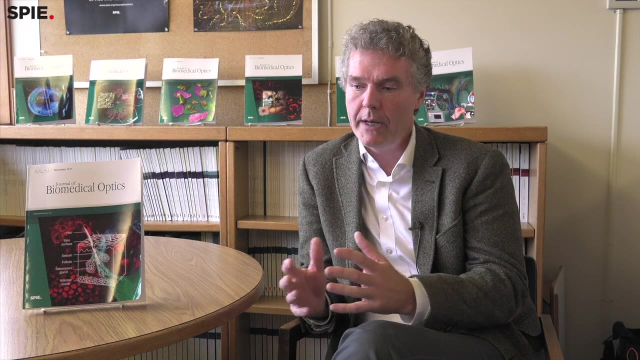 we really bridge that translational gap. I view a journal as a community, the community that brings people together. And SPIE is the community for biomedical optics. It is the single largest community in the biomedical optics world, And BIOS, the conference where we meet every January, is the venue where we present. 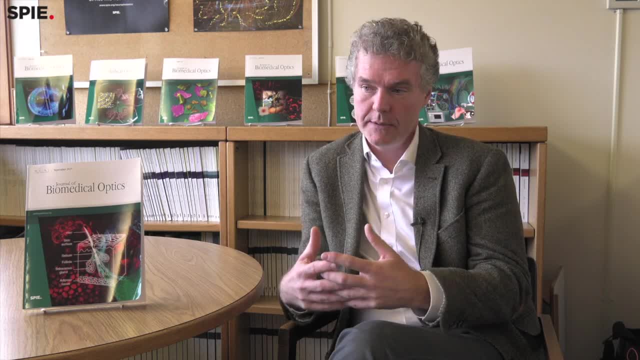 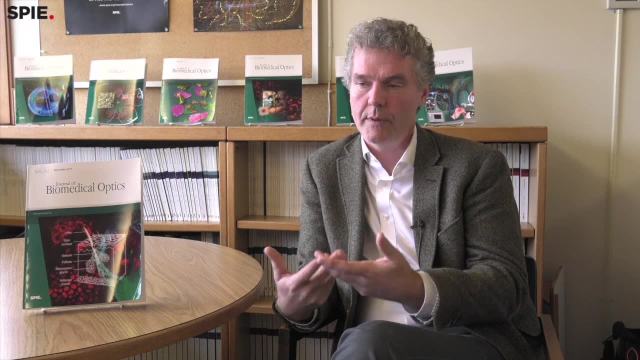 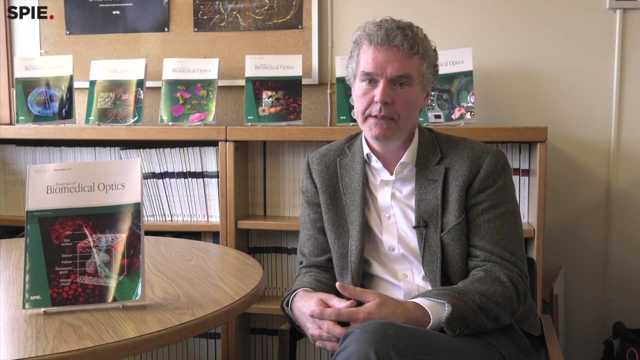 to each other And the journal biomedical optics is the issue, the paper issue or now the electronic journal that we all publish in to represent our community. So to be involved in that journal and to help it chart where it's going in the future is just a natural piece of service to the SPIE and 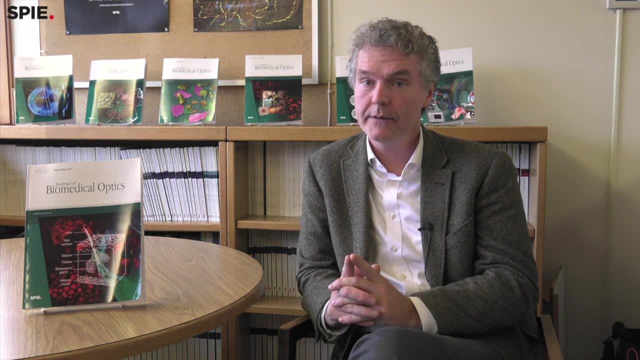 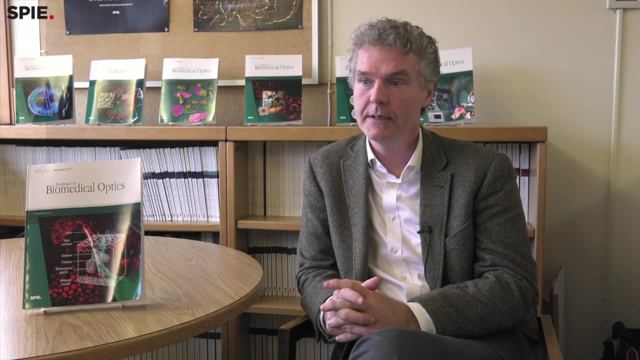 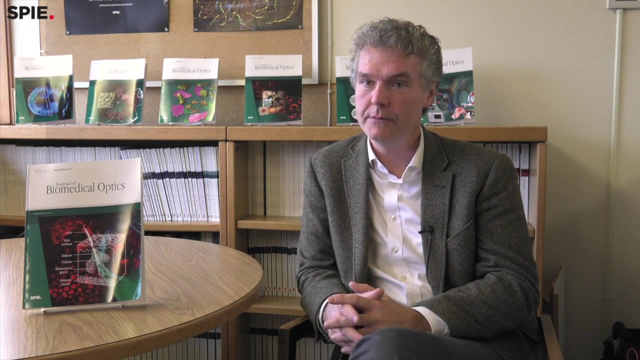 biomedical optics society. So the single biggest factor that is going to impact journal biomedical optics in the next year is this transition to open access. It will allow our papers to get viewed by everybody in the world. It's a fantastic opportunity to reinvigorate your publishing with JBL. So if you are a 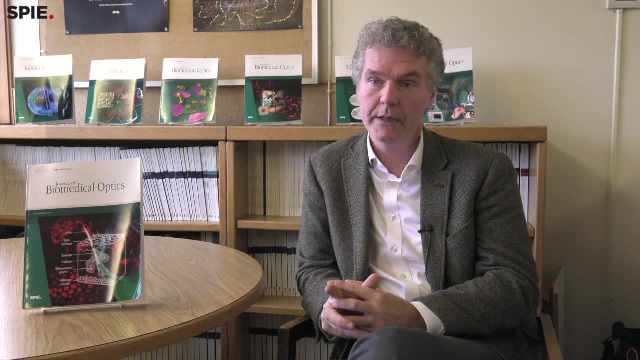 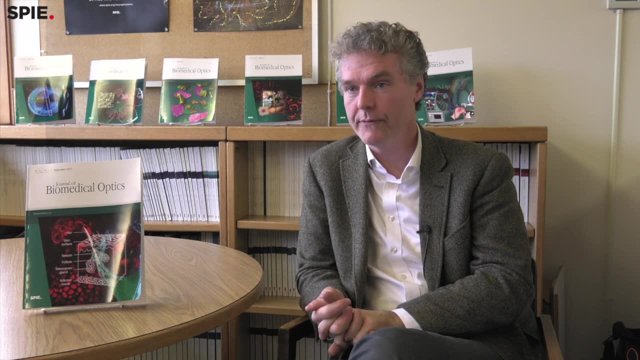 biomedical optics researcher doing translational research, working in a hospital, working in an engineering school and you have innovative discovery, you know this is the perfect time to consider publishing with the journal biomedical optics.